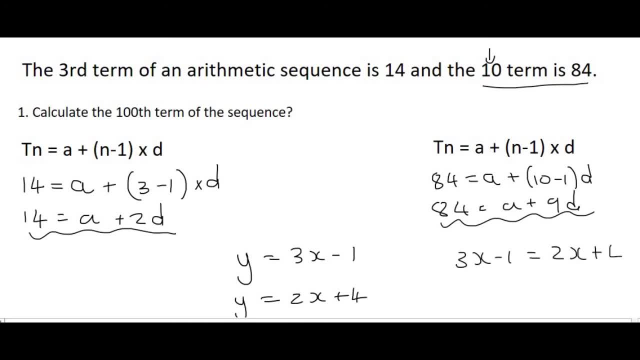 you just make them equal to each other like that. Okay, So that is correct, but you're not actually making them equal. What you're doing is a technique called substitution. So, for example, if we look at this first part here, it says that Y is the same as three X minus one. Then what we? 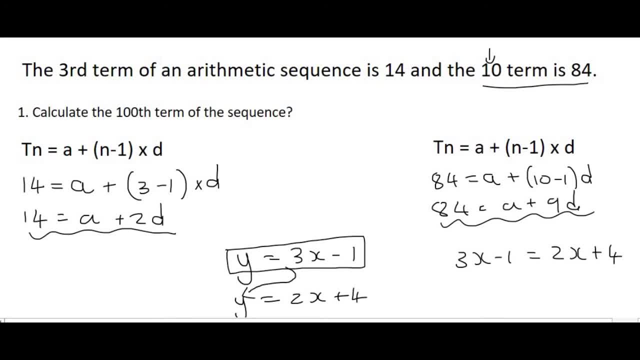 do is we go to the other equation and wherever we see a Y, we replace it with three X minus one, And so we end up with three X minus one and we get a substitution. So we end up with three X minus one equals to two X plus four. So you don't. so you're actually just replacing the one letter with. 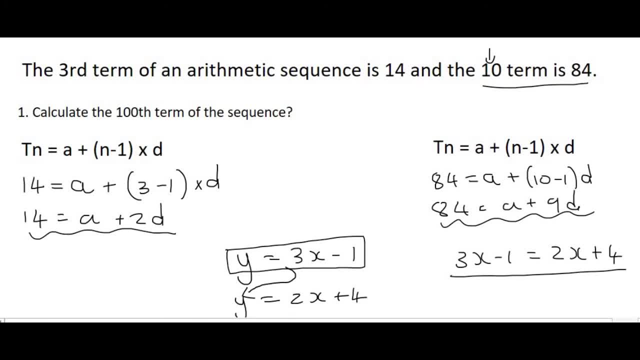 the other expression. Okay, So let's do that now in this example. So we could, for example, call this equation number one: and we need to get A or D by itself. So let's just get A by itself quickly. So that's going to give us A equals to 14 minus two D, And we could call that equation. 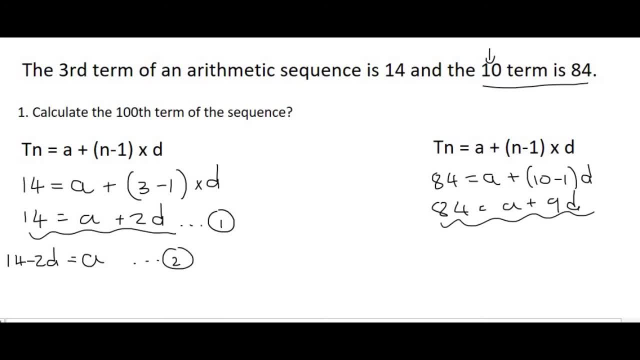 two, for example, doesn't really matter. We then take that expression and let's call this equation three. We're then going to take that equation two, and we're going to take that equation three, this expression, over here, and use that in equation number three. So what it tells us is: 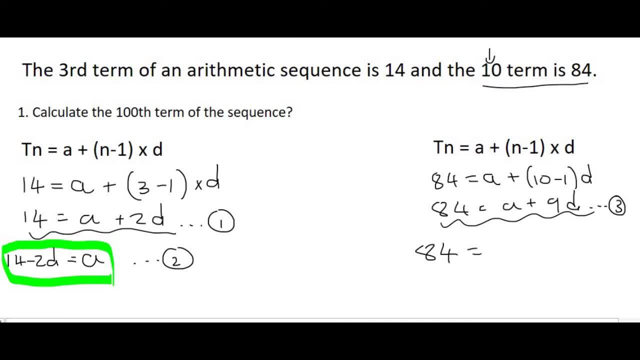 that wherever we see an A, we can replace it with 14 minus two D, like that, See, we didn't go make the equations equal to each other, And so we end up with 84 equals to 14 plus seven D. And so if 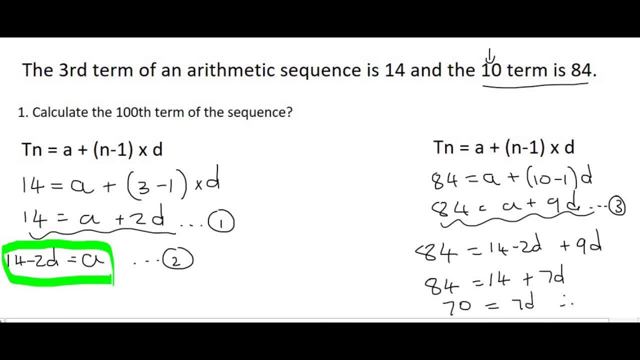 we solve for D, we get seven. D is equal to 70. Therefore, D is 10.. We then take that answer and we plug it back over here, And so we end up with A equals to 14 minus two times 10. And therefore A is going to be equal. 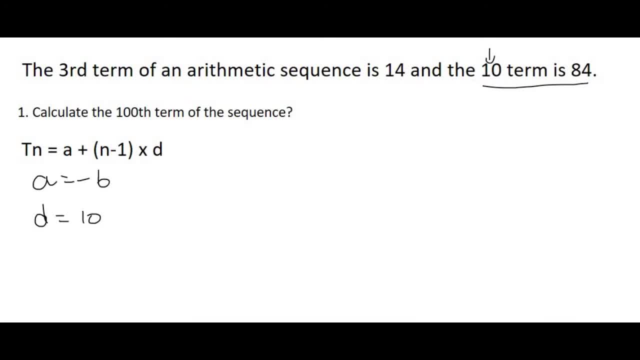 to negative six. So now we can go to. it says calculate the hundredth term, So we just go. term 100 equals two, So I'm just using the formula this one over here. So A is minus six, term 100. 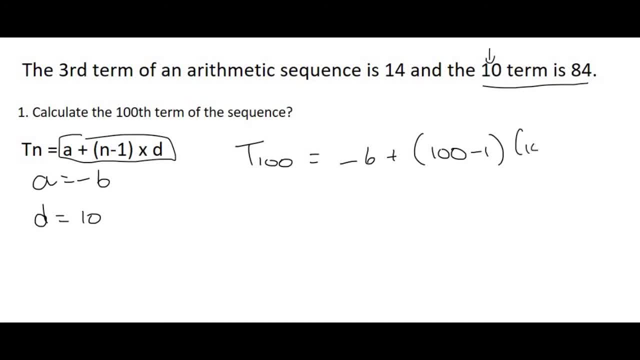 So we'll just say 100 minus one, And the common difference we just realized is 10.. Type all of this in on the calculator and you get an answer of 984.. So, guys, whenever you're doing this, whenever you get a question like this, don't try work it out in your head, Plug it into that.